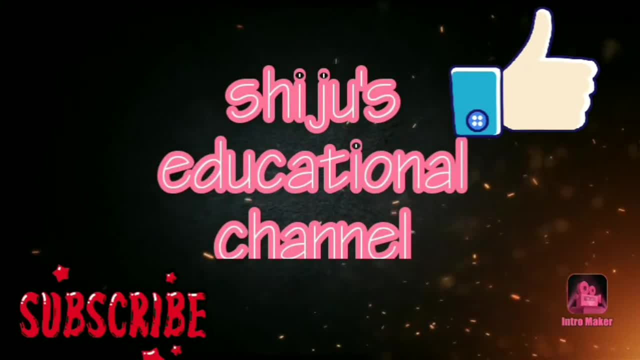 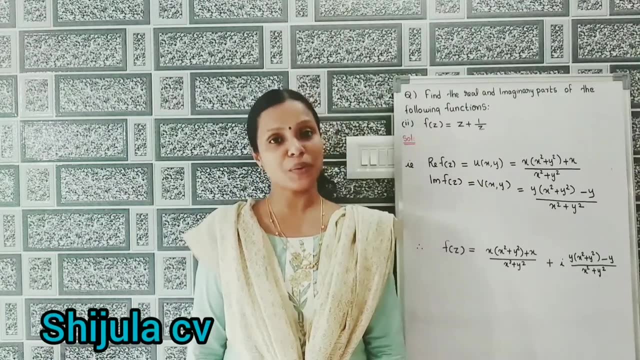 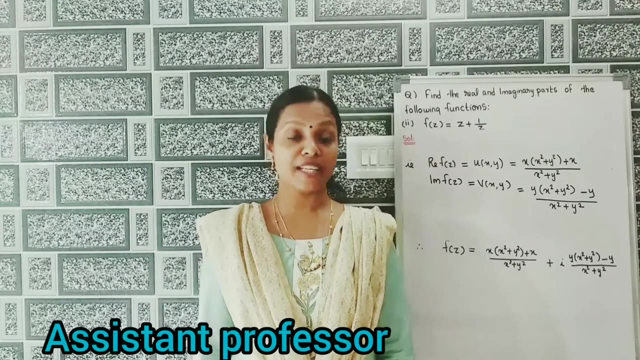 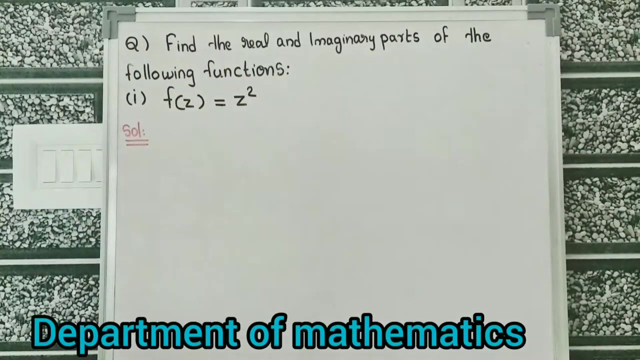 Hi everyone, welcome to the next new class and the next new session. Today we are going to learn how to find real and imaginary part of a complex function. Real and imaginary part of a complex function. Okay, let us start. Question is: find the real and imaginary parts of the following: 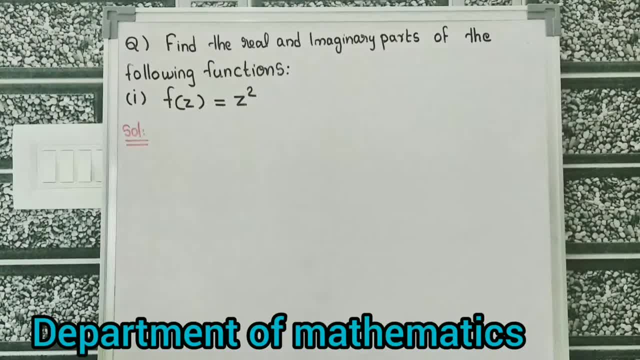 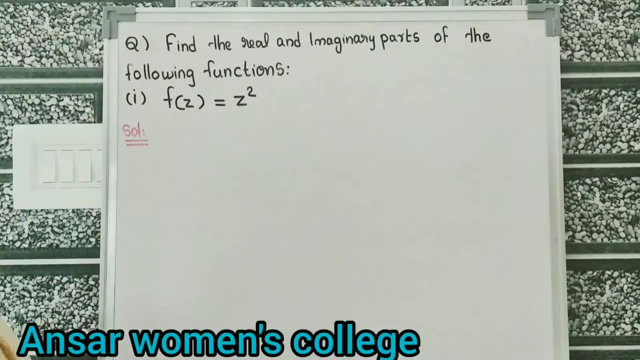 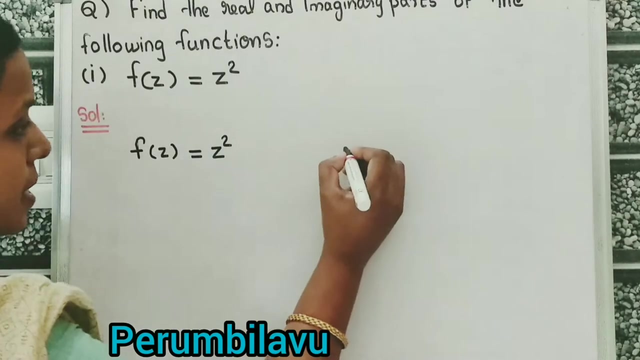 functions. Find the real and imaginary parts of the following functions Here. first question is: f of z is equal to z square. Here we have to find the real part and imaginary part of this function, that is, f of z is equal to z square. Given that f of z is equal to z square, Let us take z is. 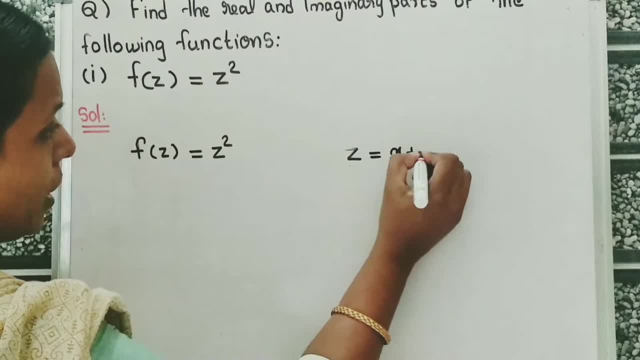 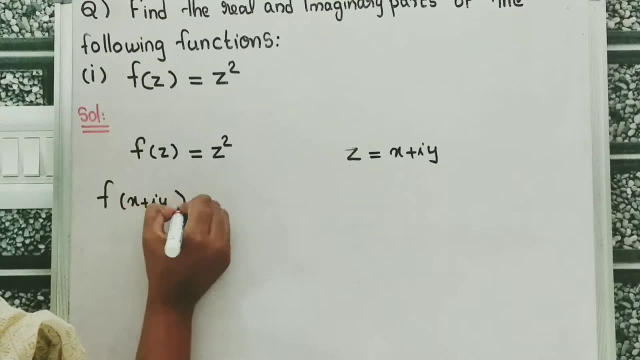 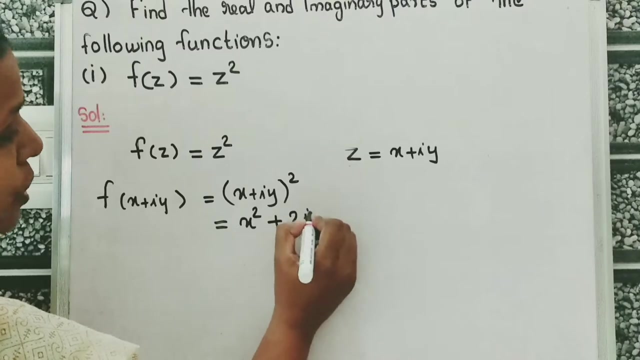 equal to x plus iy. Okay, z is equal to x plus iy. f of x plus iy equal to here: x plus iy whole square. Okay, it is of the form a plus b whole square. We can expand it as x square plus 2i into xy plus iy whole square. Okay, that is equal to. 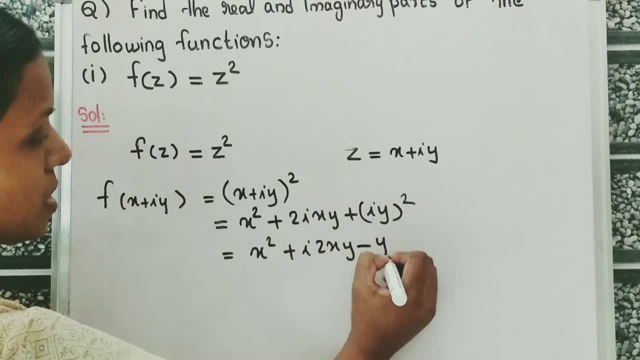 2i square plus 2i plus iy whole square. So here i square is minus 1.. We write minus y square. Okay, we get f of x plus iy is equal to x square plus i into 2xy minus y square. 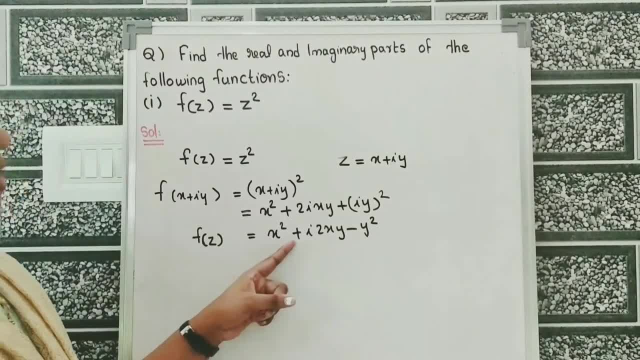 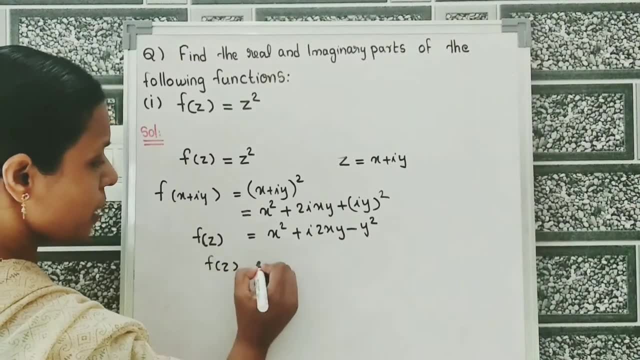 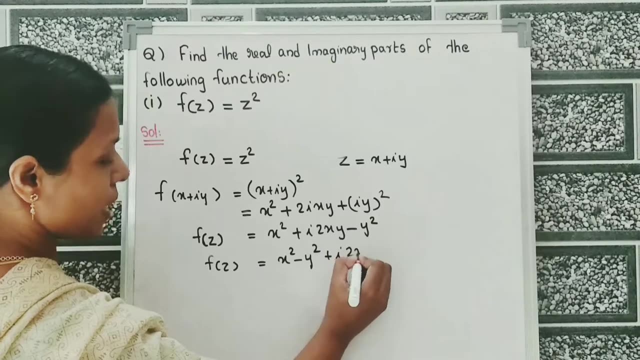 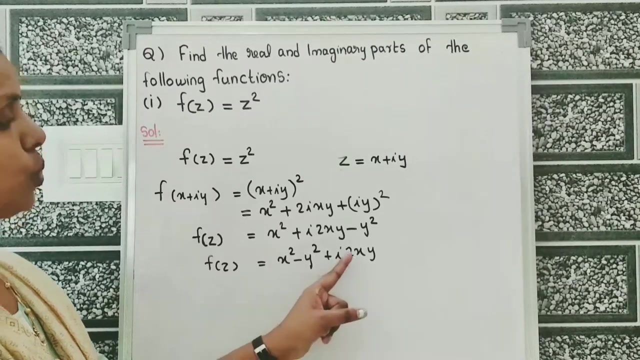 We can write: f of z is equal to x square plus i into 2xy, minus y square. Arranging this, we get f of z is equal to here: x square minus y square, Okay, plus i into 2xy. Now we get f of z is equal to x square minus y square, plus i into 2xy. It is of the form. 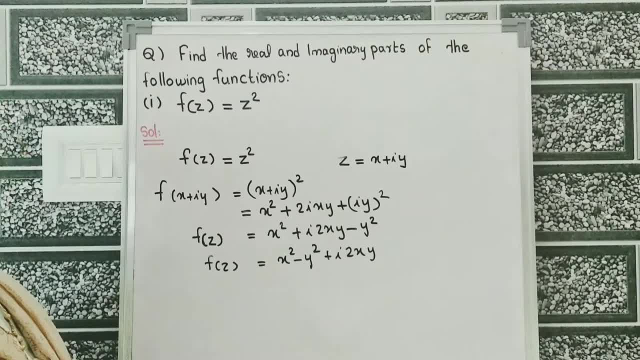 f of z is equal to u of xy plus i into v of xy. Here the real part is x square minus y square and the imaginary part is 2xy. That is, we can write: real f of z is equal to x square minus y. 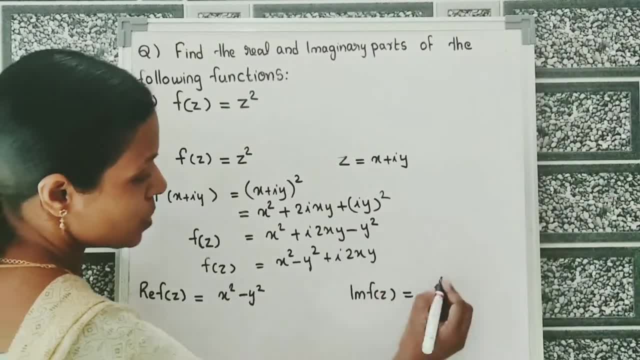 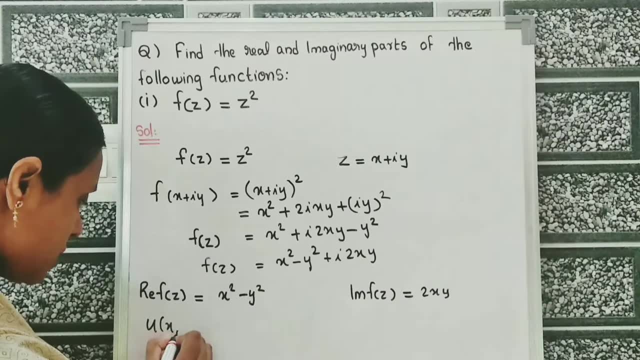 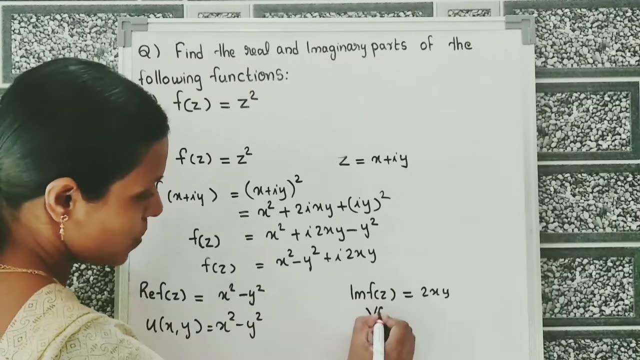 square and imaginary f of z is equal to 2xy. That is, we can real f of z is u of xy, That is, u of xy is equal to x square minus y square, and imaginary f of z is v of xy. v of xy is equal to 2xy. 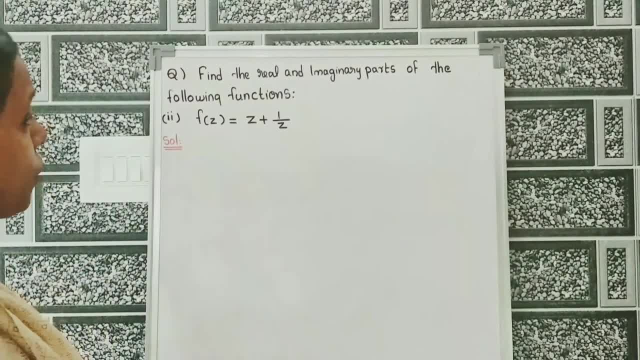 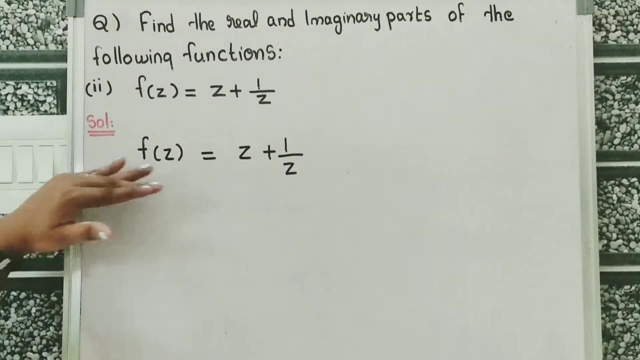 Second question is: find the real and imaginary part of this function. f of z is equal to z plus 1 by z. f of z is equal to z plus 1 by z. Here we have to find the real part and imaginary part of this function. Given that f of z is equal to z plus 1 by z, Let us take z is equal to x plus. 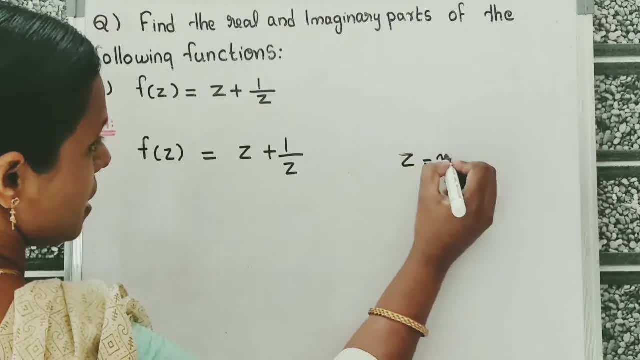 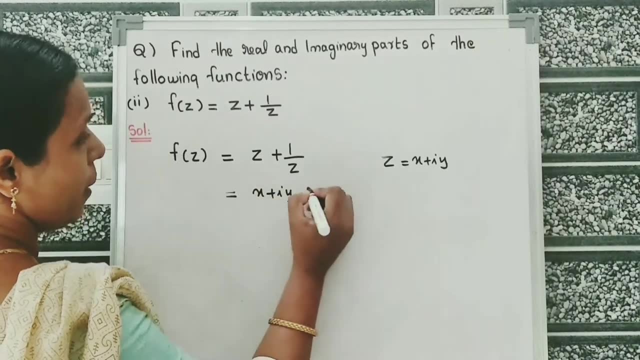 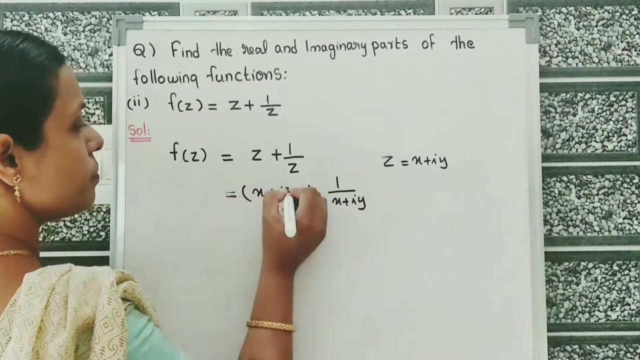 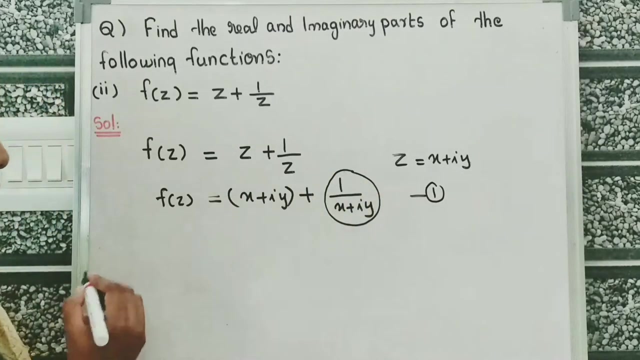 iy. z is equal to x plus iy. Putting this value in this function, we get x plus iy plus 1 by z. Here is x plus iy, x plus iy, Putting it as equation number 1.. First we arrange 1 divided by x plus iy. Here 1 divided by x plus iy equal to. we multiply numerator and denominator with its conjugate, that is x minus iy. We get 1 divided by x plus iy into x minus iy, divided by x minus iy. 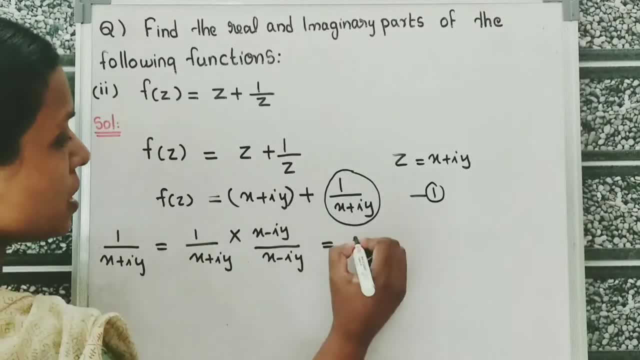 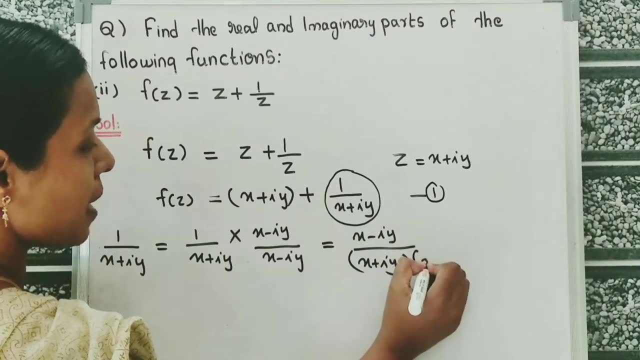 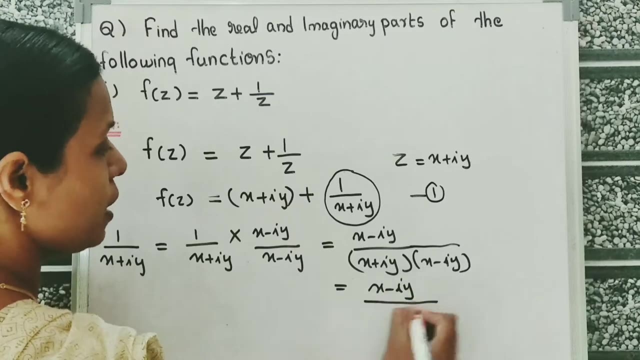 x minus iy. That is equal to: we can write x minus iy divided by here: x plus iy into x minus iy. Okay, That is equal to: we can write x minus iy divided by here: x square. It is of the form a minus b into a plus b. That is, we get a square minus b square. We get here x square plus y square. That is, we get 1 by x plus iy. 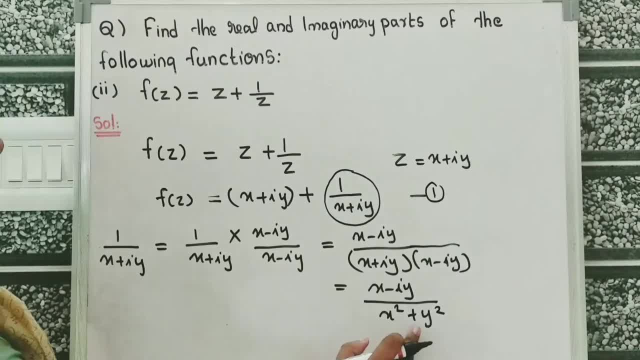 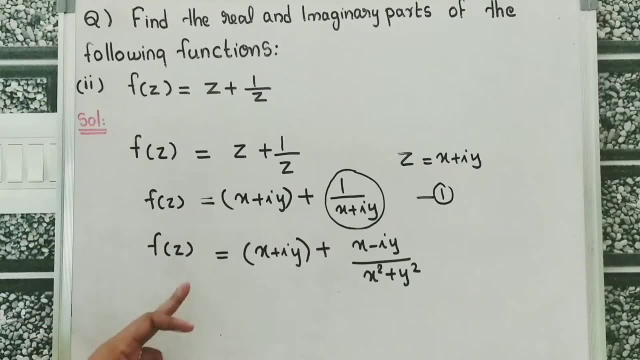 x minus iy is equal to x minus iy divided by x square plus y square. Substitute this value in equation number 1.. We get equation 1 becomes: f of z is equal to x plus iy, plus here x minus iy divided by x square plus y square. 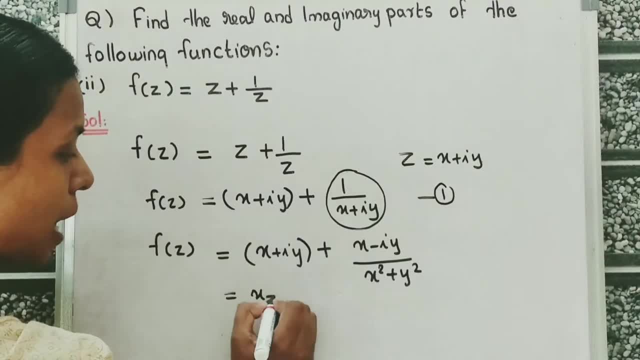 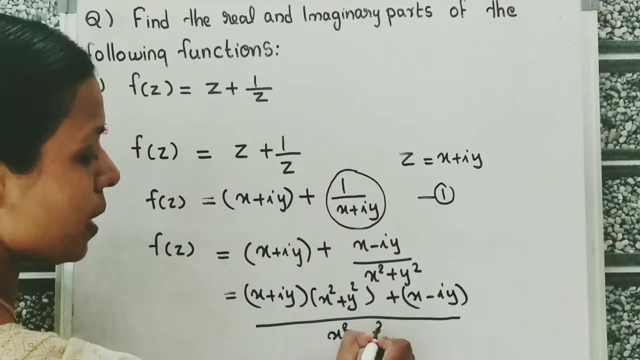 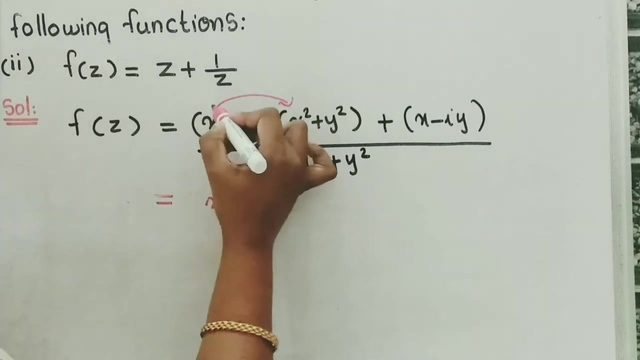 Close multiply: We get here x plus iy into x square, plus y square, plus x minus iy- Okay, All divided by x square plus y square. Here, that is equal to here: x into x square, We get x cube- Okay, x cube. and x into y square, We get plus x y square. 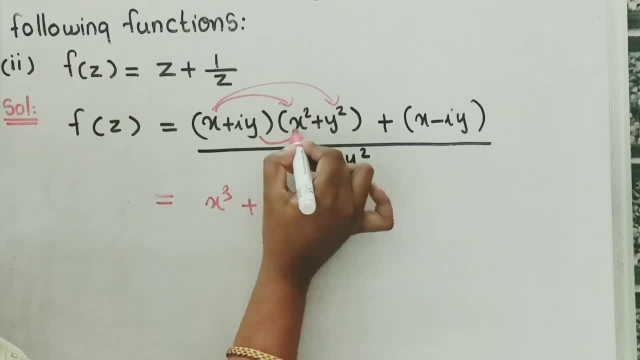 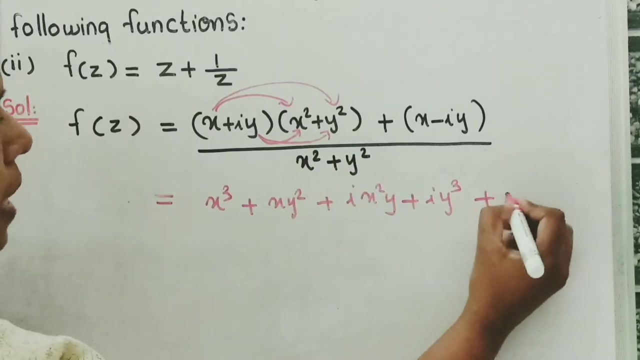 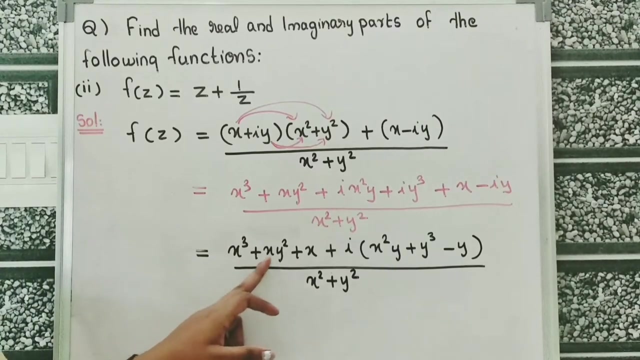 Okay. Next we multiply iy into x square. We get plus i into x square, y plus here iy into y square. We get i into y cube plus x minus iy. Okay, Divided by x square plus y square, Here separate the real part and imaginary part. We get x cube plus x y square, plus x plus i into x square, y plus y cube minus y. 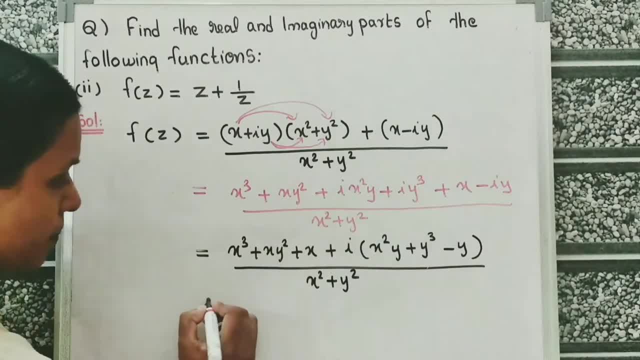 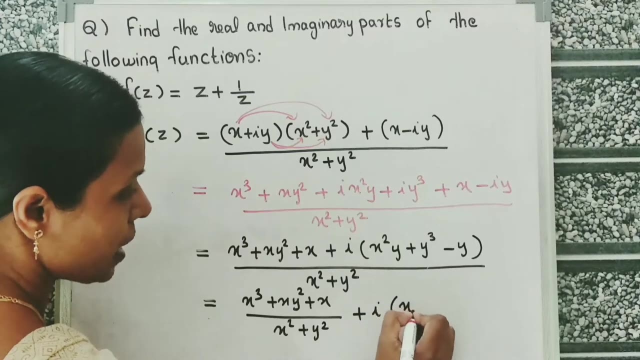 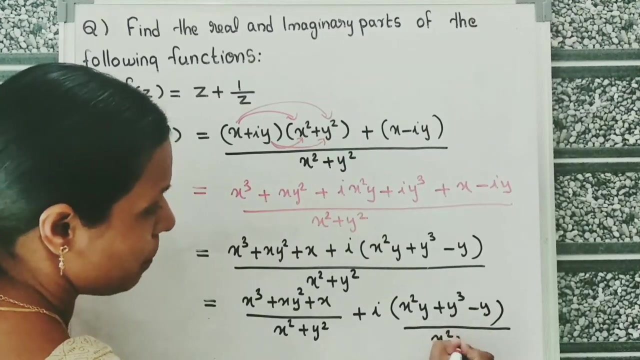 All divided by x square plus y square. Next we write Here: the real part is x cube plus x y square plus x divided by x square plus y square. Okay, Plus i into here: x square y plus y cube minus y divided by x square plus y square. 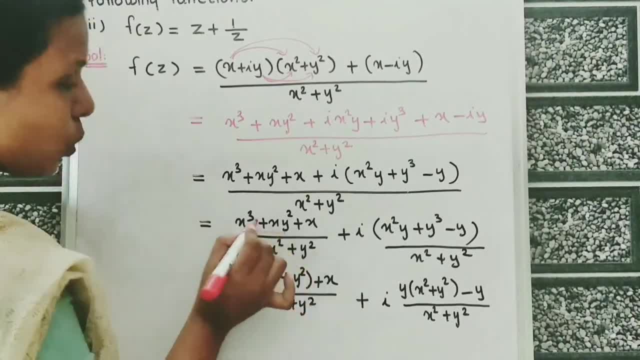 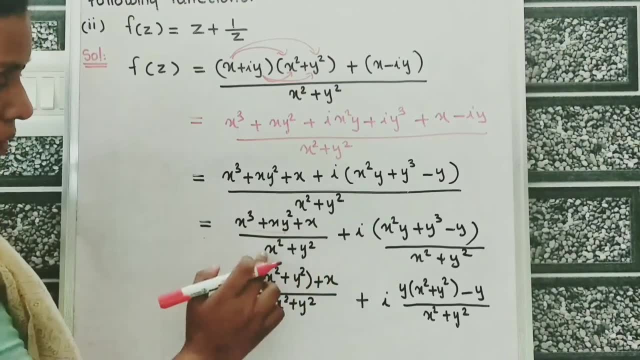 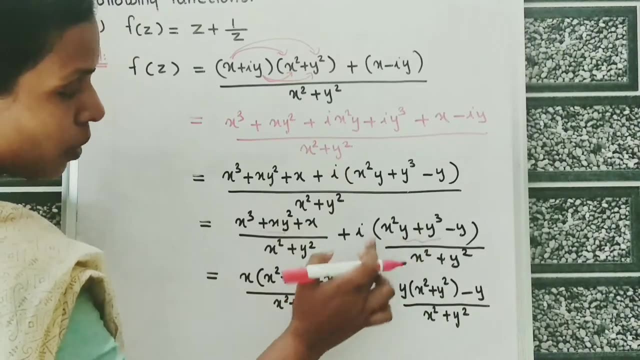 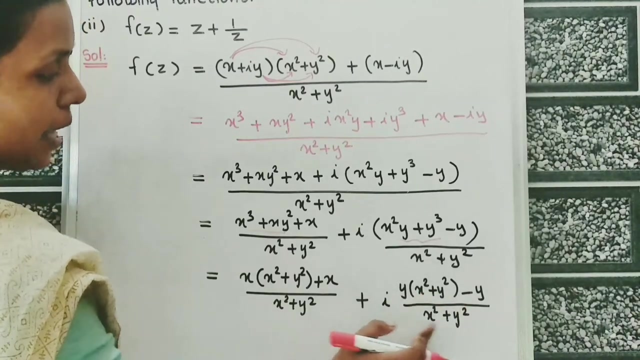 Next we write from this x cube plus x y square. Taking x outside, We get x into x square plus y square plus x divided by x square plus y square plus i into in this section we can take y outside. Then we write y into x square plus y square minus y divided by x square plus y square. 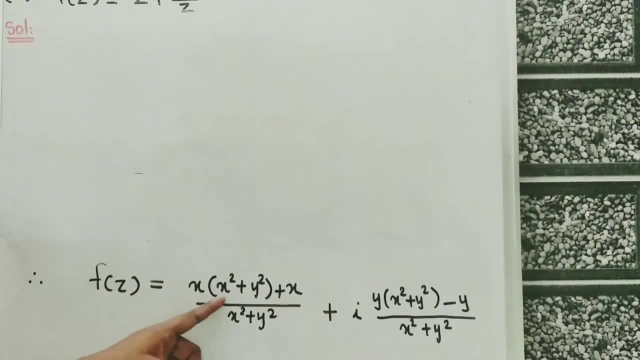 Clear. Now we get f of z is equal to x into x square plus y square plus x divided by x square plus y square plus i into y, into x square plus y square minus y divided by x square plus y square. okay, It is of the form. 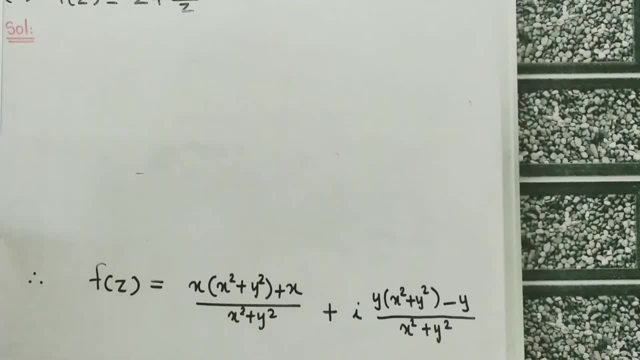 u of xy plus i into v of xy. Here the real part is this part, okay, And imaginary part is this: that is u of xy is this and v of xy is this. That is real part of f of z is re of f of z.